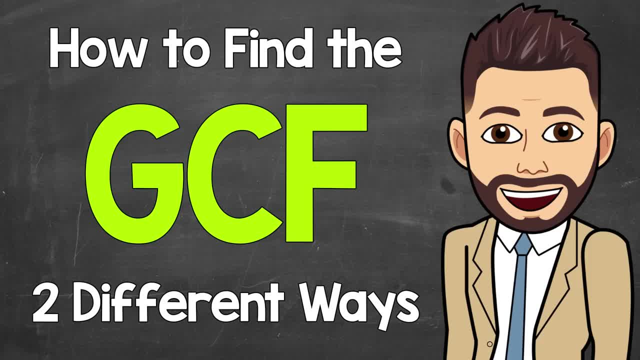 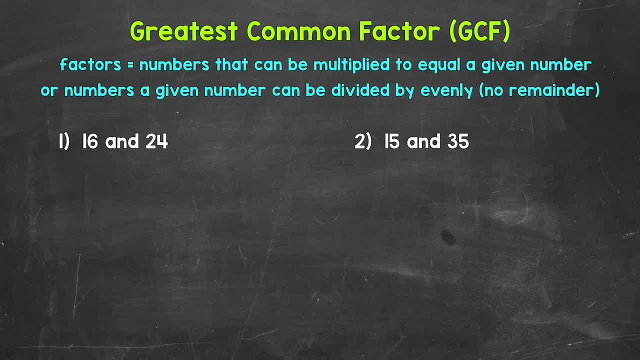 Welcome to Math with Mr J. In this video, I'm going to cover how to find the greatest common factor, also known as the GCF, using two different strategies: listing out factors and prime factorization. We're going to start by looking at the strategy of listing out. 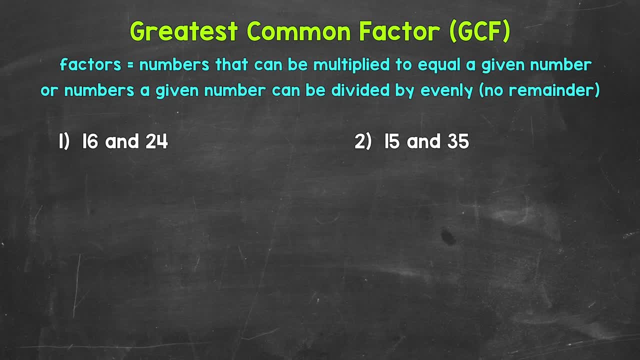 all of the factors of the numbers in order to find the greatest common factor, Then we'll move to using prime factorization. Now, as far as the greatest common factor between numbers, this is going to be the largest factor in value that both numbers share. 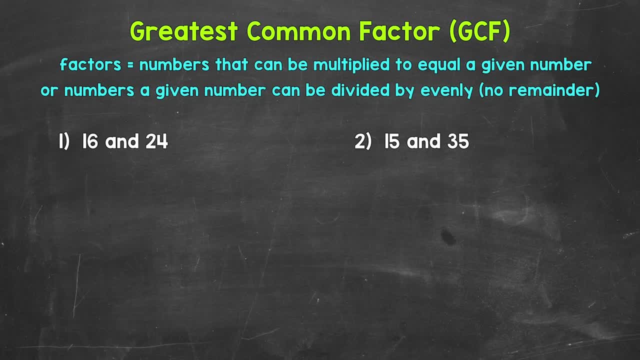 Factors are the numbers that can be multiplied to equal a given number. Or you can think of factors as the numbers a given number can be divided by evenly, so divided with no remainder. Now, it's not the most technical or mathematical way to word it, but you can think of factors as the numbers that go into the given. 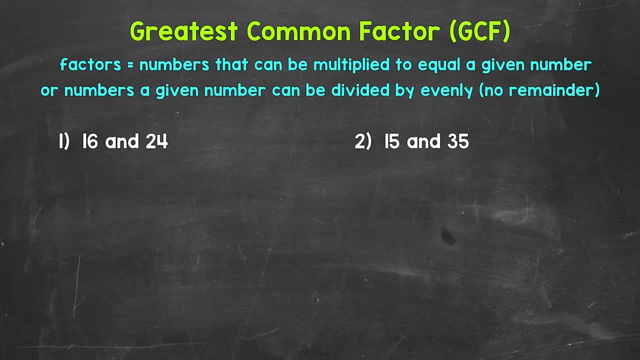 number. So, again, the greatest common factor is going to be the greatest or largest factor in value that both numbers share, that both numbers have in common. Let's jump into our examples and see exactly what this looks like, Starting with number one, where we have 16 and 24.. 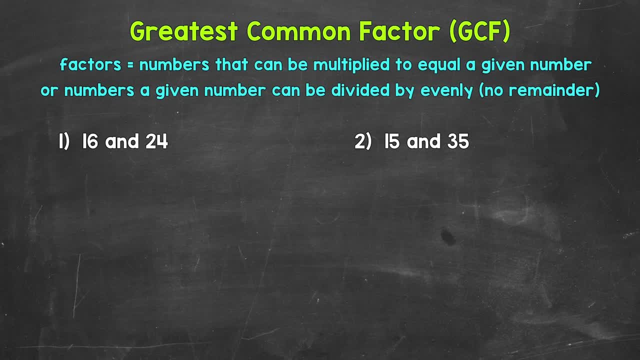 We first need to list the factors of each number. Let's start with the factors of 16.. Now I would suggest always starting with the factors of one and the number itself, because we know, one times that number will equal that number itself. 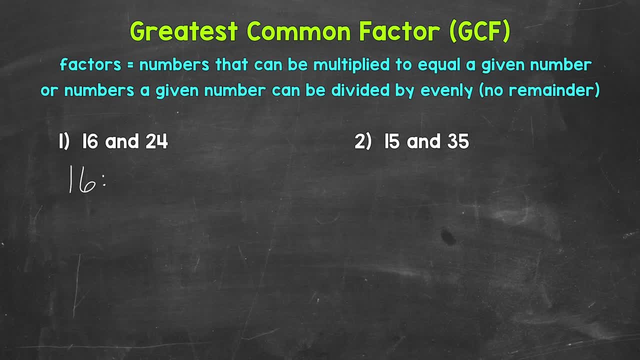 We can think of factors in terms of pairs: One times 16 equals 16.. Or we can think of it in terms of division. We can divide 16 by those factors, evenly, However you want to think about it. So I'm going to write 1 and 16, with a gap in between for the other factors. 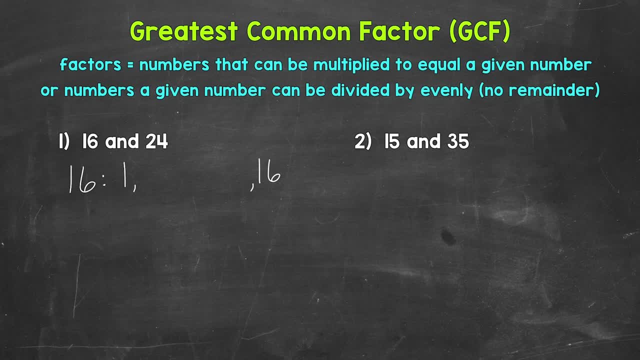 That way we can write the factors in order. Now we need to list the other factors of 16.. So let's think about what else goes into 16,, so to speak. Think about multiplication facts, division facts, and we can work our way up from 1.. 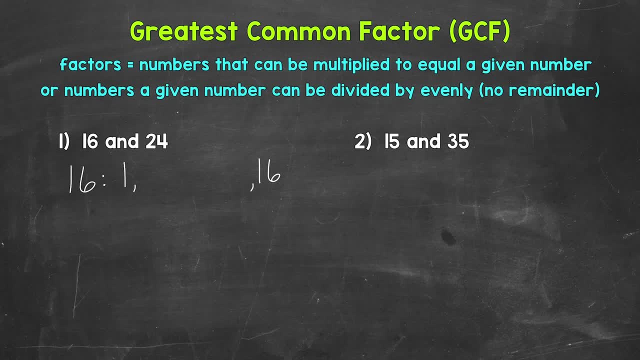 There are different strategies and ways to work through the please Next 그것es. The next factors of 16 means two and eight. 2 times 8 equals 16.. So 2 and 8 are factors of 16.. Now let's use a mouse. 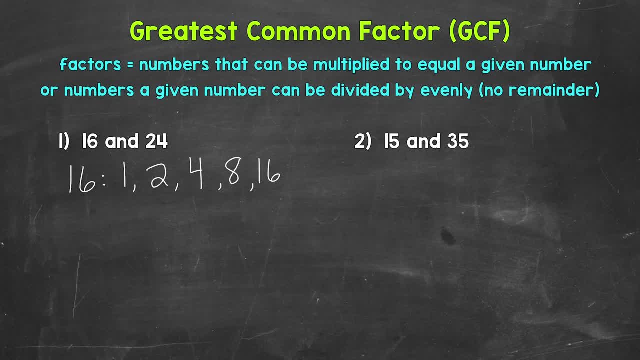 Now this is our last factor of 16 we'll use for the graph: 2 times 4 equals 4, code 16.. Breast cancer is a factor of 16.. of 16.. Although 4 times 4 equals 16, we only need to write 4 once in our factors list. 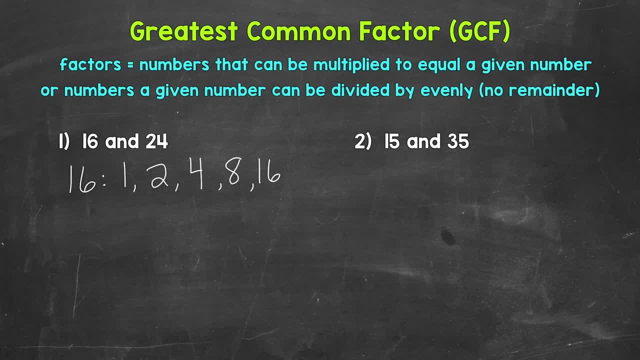 And that's it for the factors of 16.. You can always think about other possible factors if you're unsure, if you're done, For example, 3, 5,, 6, and so on. But we have them all. The factors of 16 are 1,, 2,, 4,, 8, and 16.. Let's move on to the factors of 24.. We will start with. 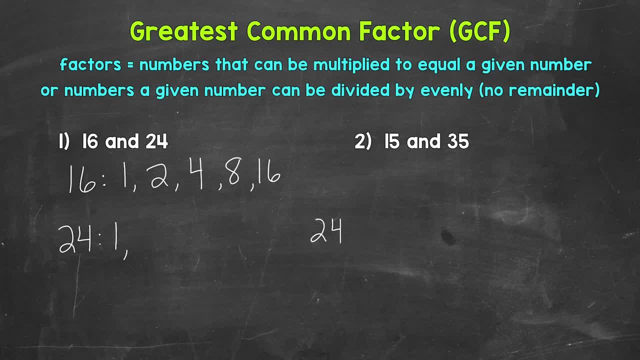 1 and 24.. Next we have 2 and 12.. 2 times 12 equals 24.. So 2 and 12 are factors of 24.. Then we have 2 and 12 equals 24.. So 2 and 12 are factors of 24.. Then we have: 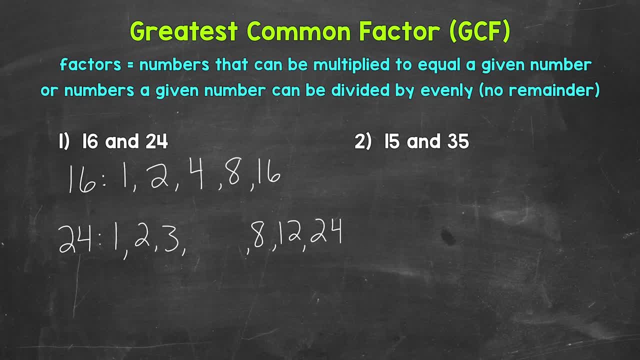 2 and 12 equals 24.. So 2 and 12 are factors of 24.. Then we have 3 and 8.. 3 times 8 equals 24.. So 3 and 8 are factors of 24.. 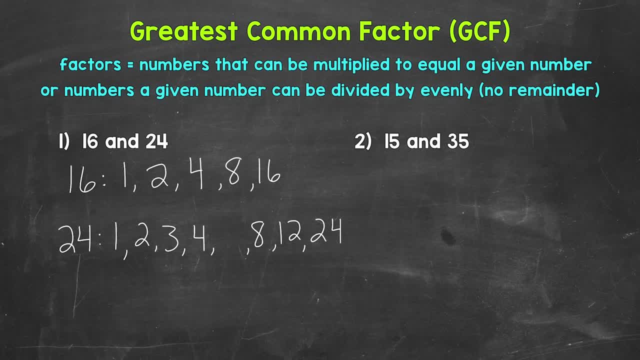 And then, lastly, we have 4 and 6.. 4 times 6 equals 24.. So 4 and 6 are factors of 24.. And that's it for the factors of 24.. 1,, 2,, 3,, 4,, 6,, 8,, 12, and 24.. 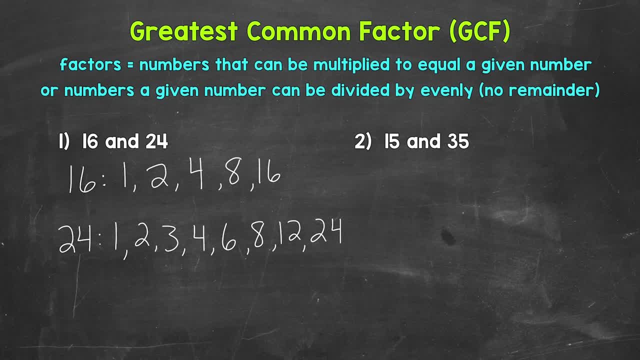 Now that we have the factors listed for our numbers, we need to look for common factors and specifically, the greatest common factor. So let's look for factors that these numbers share, that they have in common. So 1 is a common factor, 2 is a common factor, 4 is a common factor. 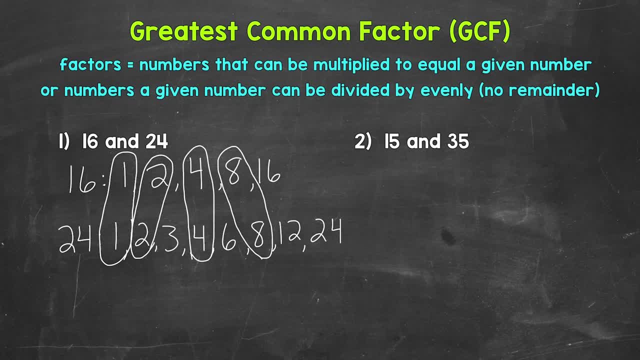 And then 8 is a common factor. So the greatest common factor is 8.. The greatest factor in value that they share, The greatest factor in value that they have in common, So the GCF, the greatest common factor, is 8.. The greatest common factor of 16 and 24 is 8.. 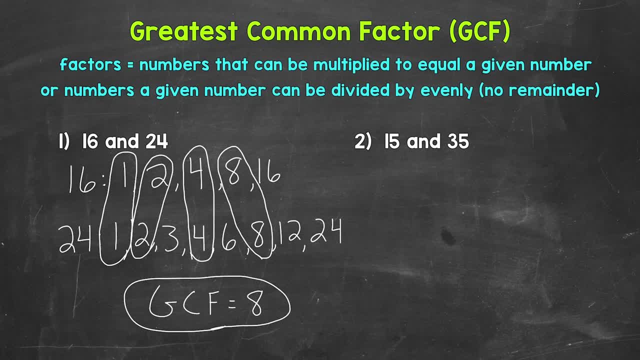 Let's move on to number 2, where we have 15 and 35.. Let's start with the factors. We have 1 and 15.. We have 1 and 15.. Next we have 3 and 5.. 3 times 5 equals 15.. So 3 and 5 are factors of 15.. 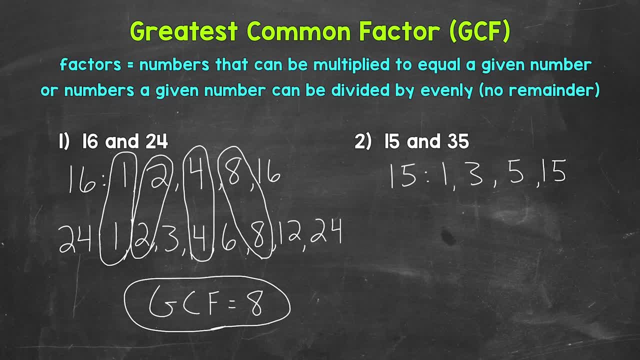 And that's it for the factors of 15.. 1, 3,, 5, and 15.. Now let's list the factors of 35. So we have 1 and 15. 1 and 35. And then 5 and 7. 5 times 7 equals 35. So 5 and 7 are factors of 35.. 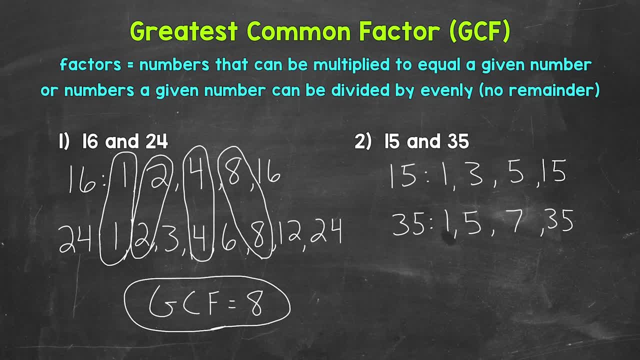 And that's it for the factors of 35.. 1,, 5,, 7, and 35.. Now that we have our factors list for our numbers, we need to look for common factors and specifically the greatest common factor. So 1 is a common factor. 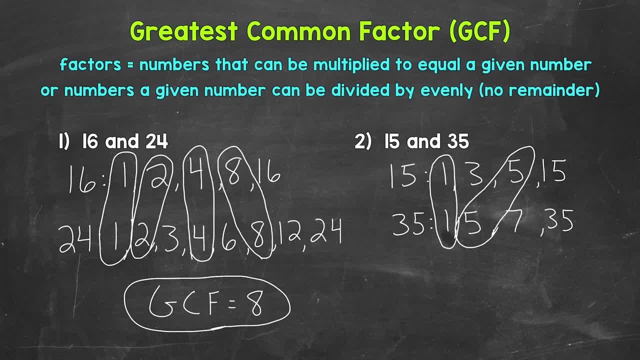 And then 5 is a common factor. That means 5 is the greatest common factor. So the GCF, the greatest common factor, is 5.. The greatest common factor of 15 and 35 is 5.. So there's how we list factors in order to find the greatest common factor. 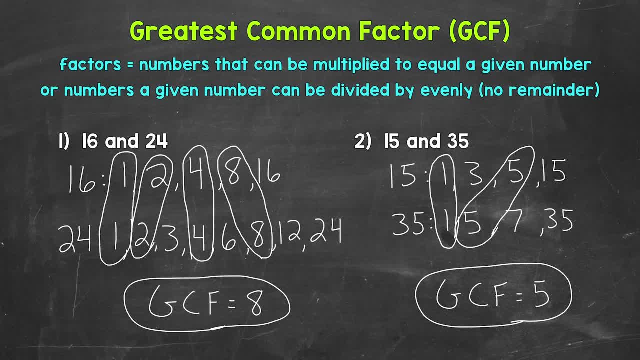 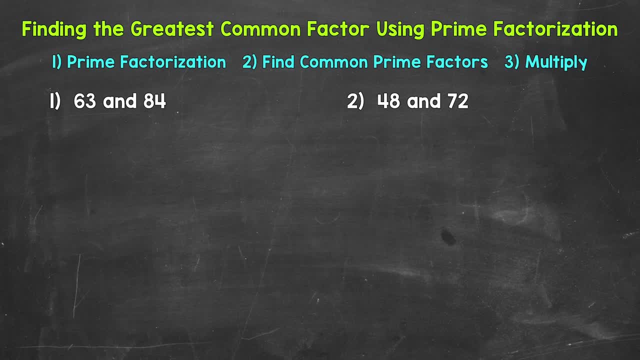 Let's move on to using prime factorization. Here are our examples For using prime factorization Now. I like using this strategy and find it helpful when working with numbers that are a little larger in value and not as simple to work with, For example. 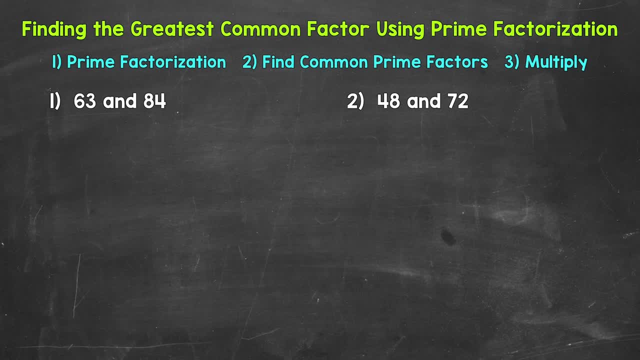 the strategy of listing out all of the factors of the numbers in order to find the GCF can be kind of difficult and time-consuming when working with larger numbers in value. So this is a different approach, a different strategy to be familiar with when it comes to finding the greatest common factor. 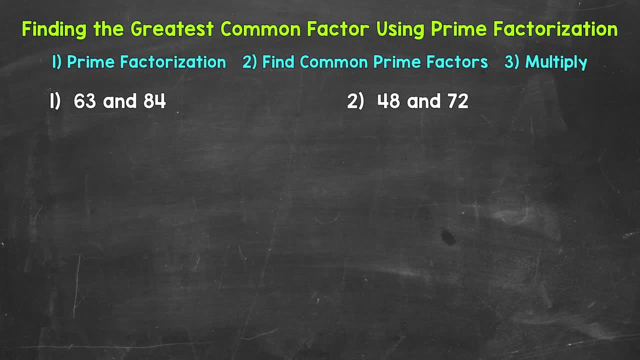 Let's jump into our examples, starting with number 1, where we have 63 and 84.. Let's start with the prime factorization of 63. And we will start with the factors of 7 and 9.. 7 times 9 equals 63. So 7 and 9 are factors of 63. 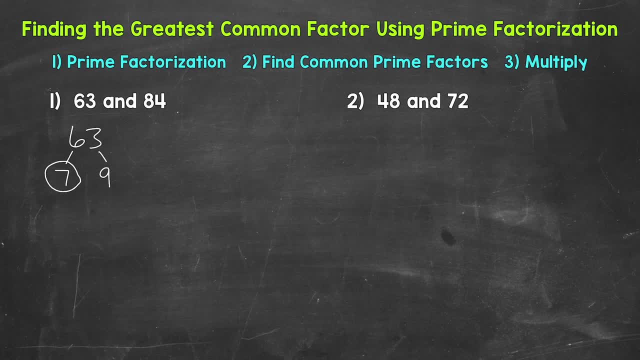 7 times 9 equals 63. So 7 and 9 are factors of 63.. 7 times 9 equals 63.. So 7 and 9 are factors of 63.. Now 7 is prime. so we are done there. 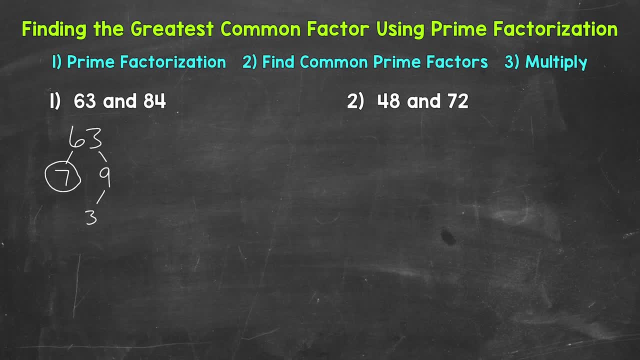 9. we can break down: 3 times 3 equals 9.. So 3 is a factor of 9.. 3 is prime. So we are done there and there, And that's the prime factorization of 63. We can't break that down any further. 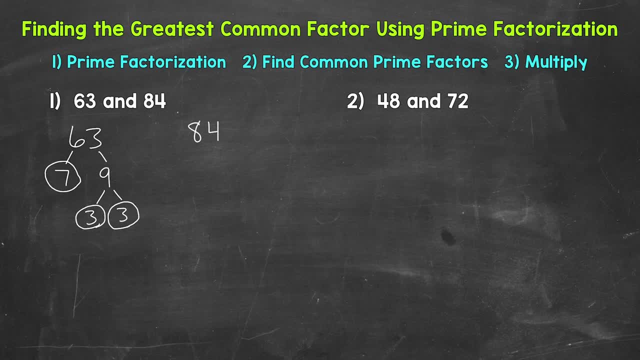 Now we have the prime factorization of 84.. Let's start with the factors of 2.. 2 and 42.. 2 times 42 equals 84. So 2 and 42 are factors of 84. Now 2 is prime. so we are done there. 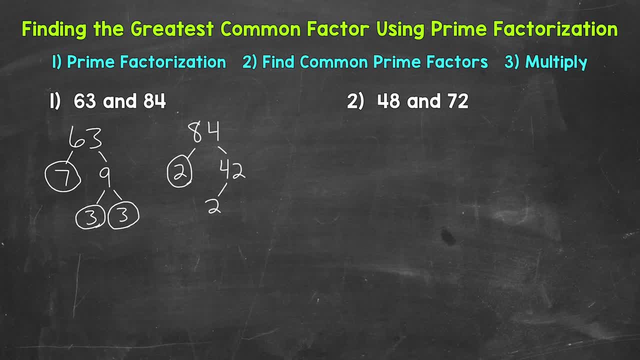 42, we can break down 2 times 21, equals 42. So 2 and 21 are factors of 42.. 2 is prime, so we are done there. 21, we can break down 3 times 7, equals 21.. So 3 and 7 are factors of 21.. 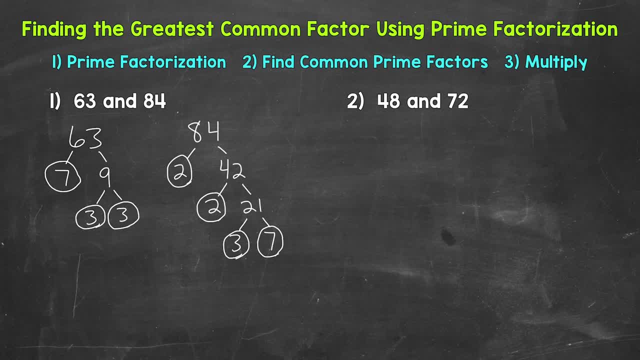 3 is prime and 7 is prime as well. So we are done. That's the prime factorization of 84.. We can't break that down any further Now that we have the prime factorization of both of those numbers. 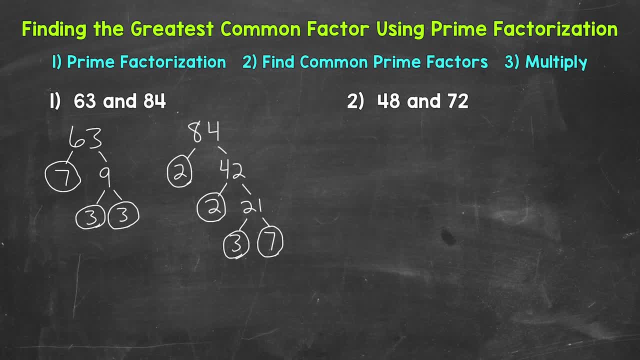 we need to find common prime factors, So prime factors that they share. Now I'm going to list the prime factors of each to make it easier to find the ones they have in common. So, as far as 63,, we have 3,, 3, and 7.. 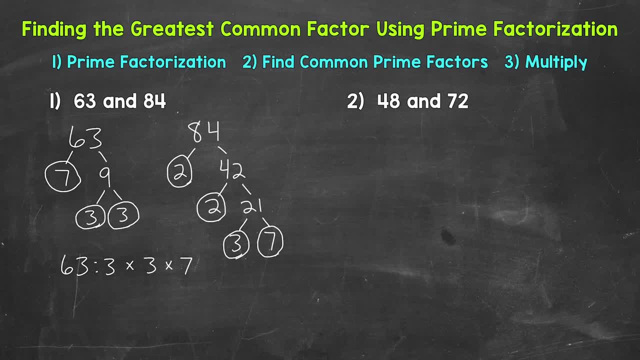 3 times 3 times 7 equals 63.. For 84,, we have 2,, 2,, 3, and 7.. 2 times 2 times 3 times 7 equals 84.. Now we need to find any common prime factors. 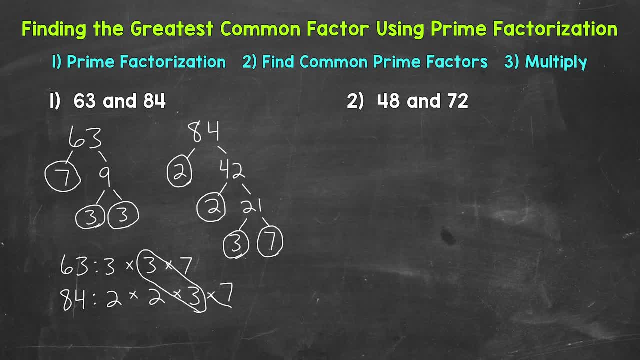 3 is a common prime factor And 7 is a common prime factor. So they have a 3 and a 7 in common. Once we find those common prime factors, we multiply them. So 3 times 7 equals 84.. 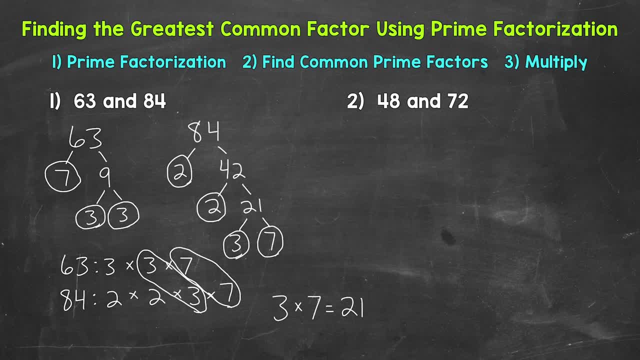 And that equals 21.. And that's our greatest common factor. So the GCF, the greatest common factor of 63 and 84, is 21.. Let's move on to number 2, where we have 48 and 72.. 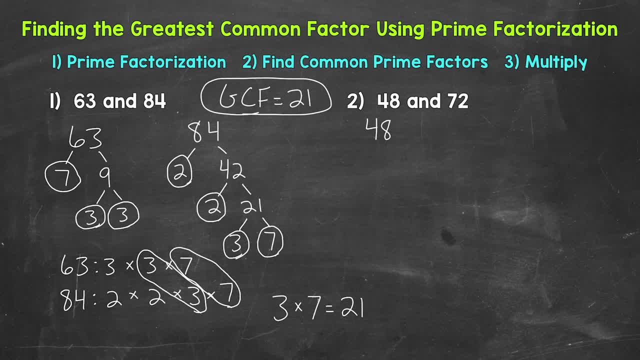 Let's start with the prime factorization of 48. And we will start with the factors of 2 and 74.. Let's start with the prime factorization of 48. And we will start with the factors of 2 and 74.. 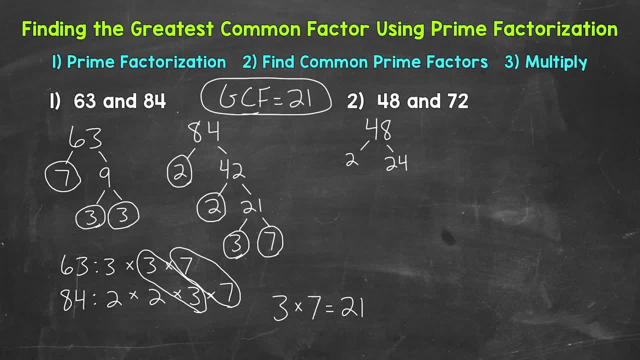 Let's start with the prime factorization of 48.. and 24.. 2 times 24 equals 48,, so they are factors. Now, 2 is prime, so we are done there. We can break down 24.. 2 times 12 equals 24,, so 2 and 12 are factors. 2 is: 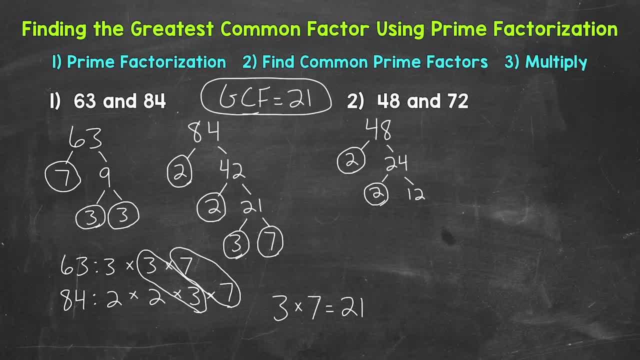 prime, so we are done there. We can break 12 down further. 2 times 6 equals 12, so 2 and 6 are factors. 2 is prime, so we are done there, but we can break 6 down. 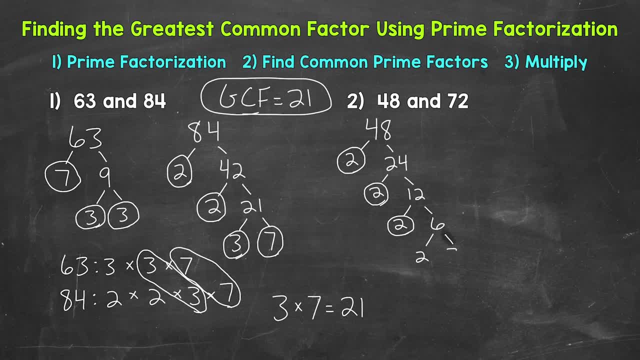 further: 2 times 3 equals 6, so 2 and 3 are factors. 2 is prime, so we are done there, And 3 is prime, so we are done there as well, And we are done with the. 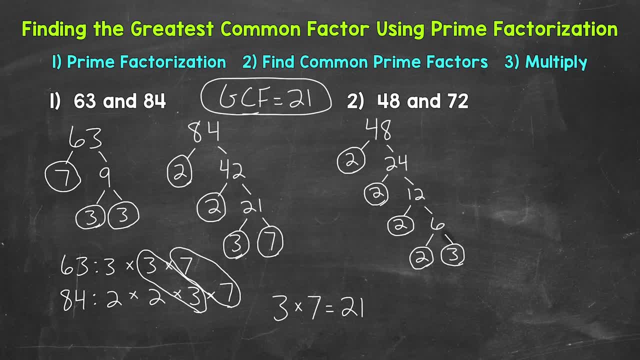 prime factorization of 48.. We can't break that down any further. Now we need the prime factorization of 48.. We can't break that down any further. Now we need the prime factorization of 72.. Let's start with the factors of 2 and 36.. 2 times. 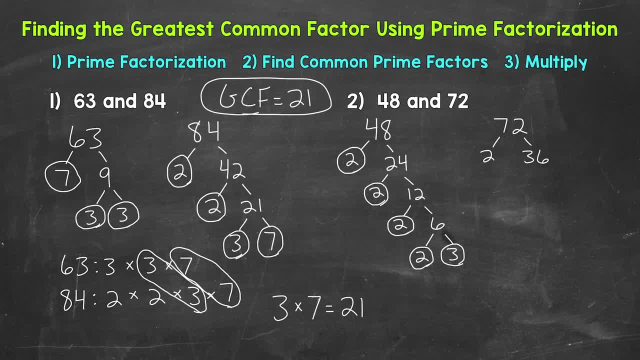 36 equals 72, so they are factors. 2 is prime, so we are done here. 36, we can break down 2 times 18, equals 36, so 2 and 18 are factors. 2 is prime, so we are done. 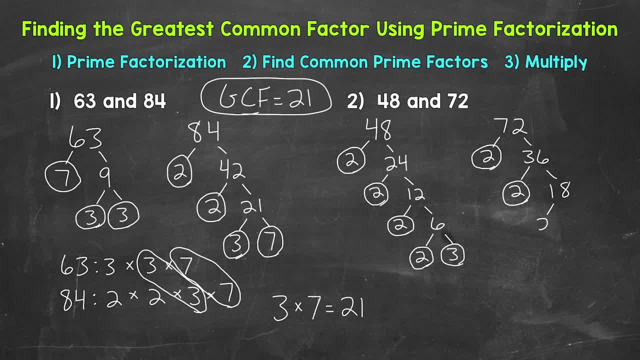 there 18. we can break down 3 times 9 equals 18, so 2 and 9 are factors. 2 is prime, so we are done there. but we can break 9 down further 3 times 3 equals 9, so 3 is a factor of 9.. 3 is prime, so we are. 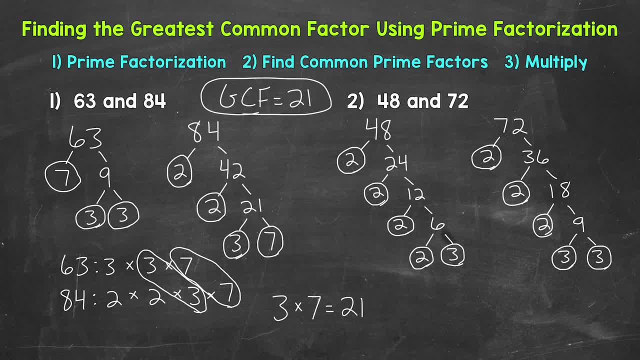 done there and there And we are done with the prime factorization of 72.. We can't break that down any further. Now that we have the prime factorization of both 72 and 3, we need to find common prime factors. So I am going to write the prime factors of 48. 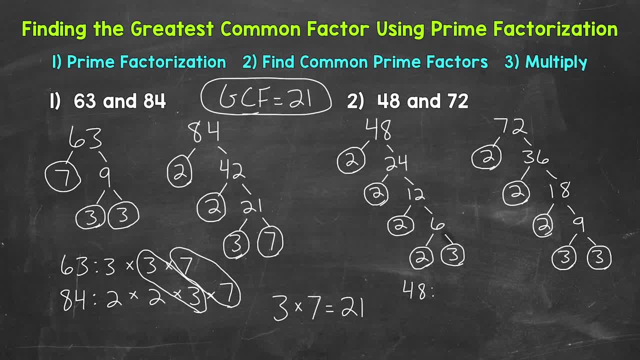 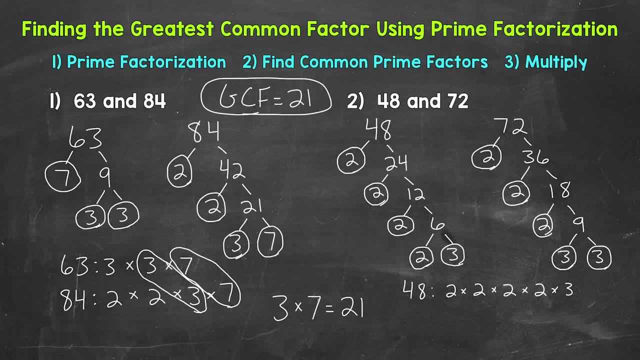 of 48 and 72. That way it is a little easier to find common prime factors. So for 48, we 3 equals 48.. For 72 we have 2, 2,, 2, 3, and 3.. 2 times 2 times 2 times 3 times 3. 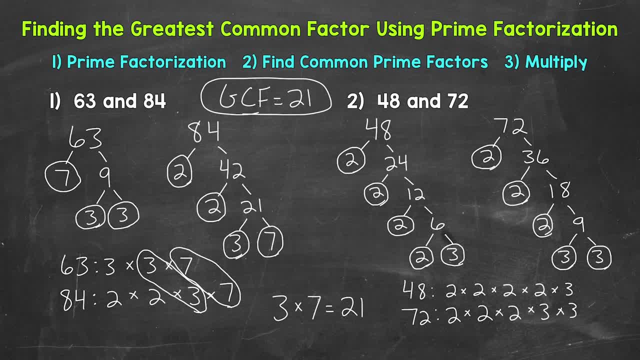 equals 72.. Now we need to find common prime factors. They have a 2 in common, another 2 in common, another 2 in common and then a 3 in common. So now that we found the common prime factors, we need to multiply them to get the greatest.